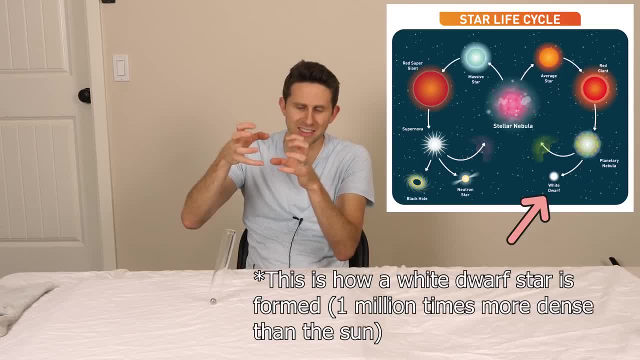 then the mass will keep collapsing in on itself in the star and it'll collapse more and more and more and more, until actual electricity Electrons are becoming so close together that they become as close together as they can possibly get, And the only thing that's stopping them from overlapping each other is the Pauli Exclusion Principle. 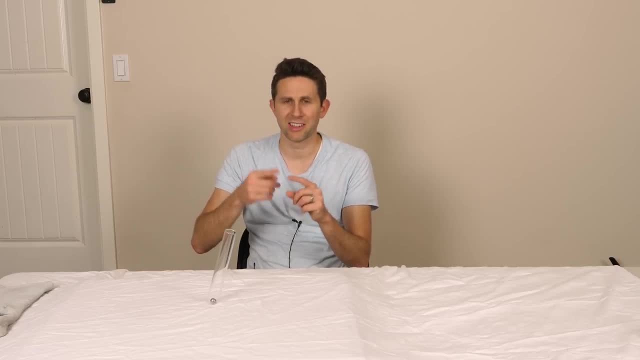 And the Pauli Exclusion Principle says that you can't have two electrons in the same place, at the same time, in the same state. But what happens if you try to force them more and more together is the only thing that's holding them apart is due to the Pauli Exclusion Principle. But it doesn't stop there. If you have too much mass still wants to attract each other, and not even the Pauli Exclusion Principle can keep the electrons from getting closer together. So as it keeps compressing stronger and stronger together, the electrons and the protons get so close together that you have electron capture. 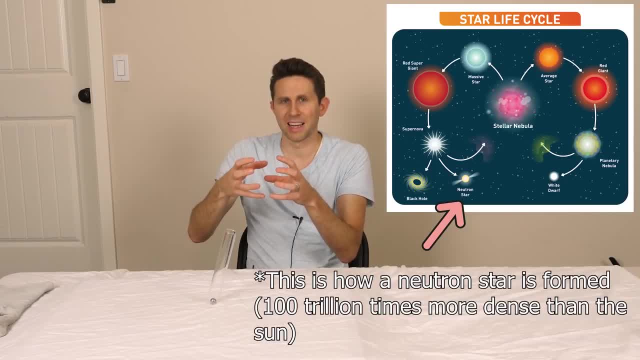 and it turns a proton and electron into a neutron And you end up with a pure neutron soup And that's called a neutron star. And it's so dense because you no longer have these protons and electrons, but you have just pure neutrons with no electrons. 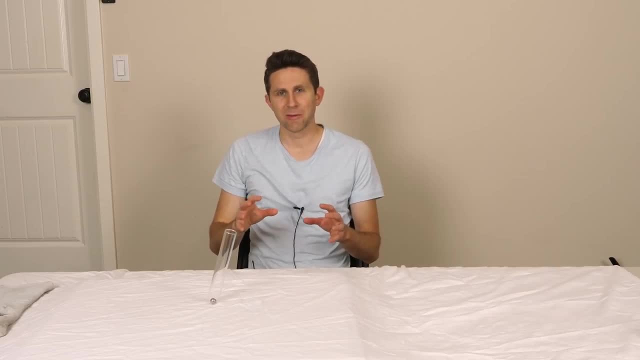 And that's called an electric charge that can come very close together. So today I want to show you what would happen if you had just a very tiny drop of a neutron star and brought it on Earth. So I have here a magic cube, And what's cool about this cube is we can. 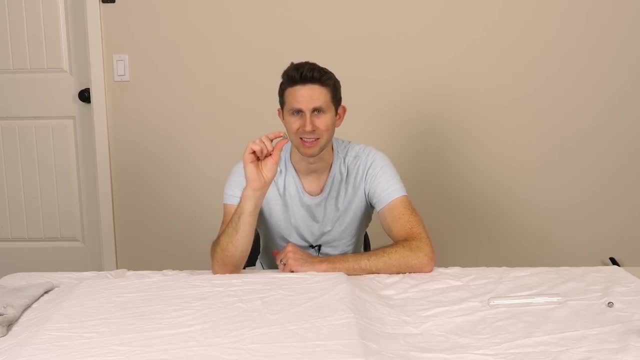 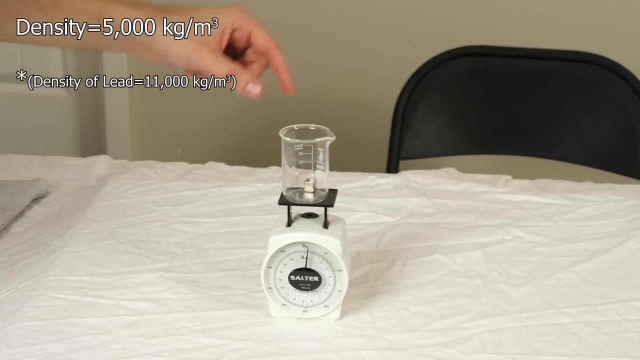 increase the density up to the density of a neutron star and see what happens. So, to start off, let me show you what it looks like. So I have a cube here, just at normal Earth density. Put it on there. Now I'm going to do my magic, touch on this cube. 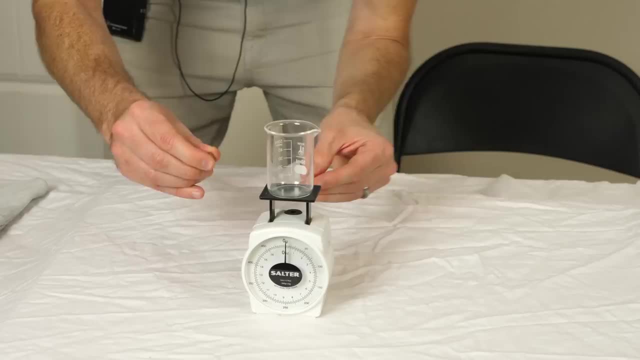 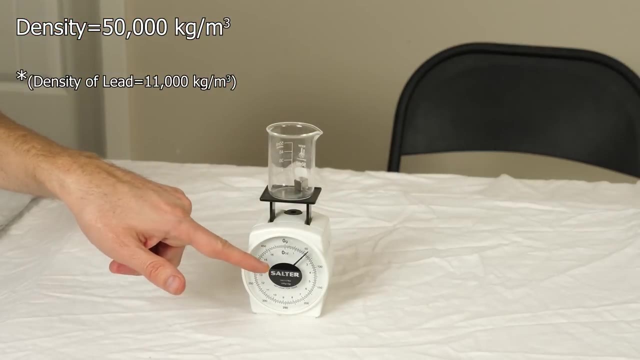 So now this is getting really heavy for the size of it. Now you can see how heavy it is. Put it in there: Weighs 50 grams instead of five. Okay, now let's increase the density even more And go. 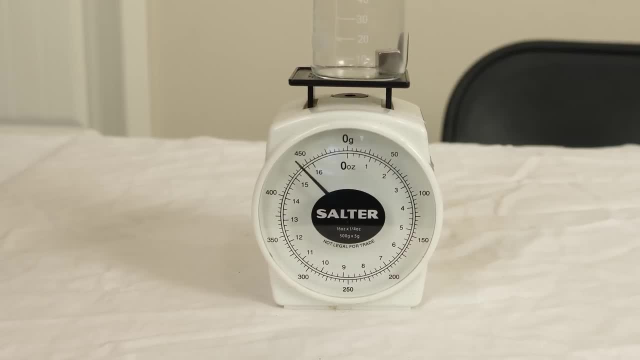 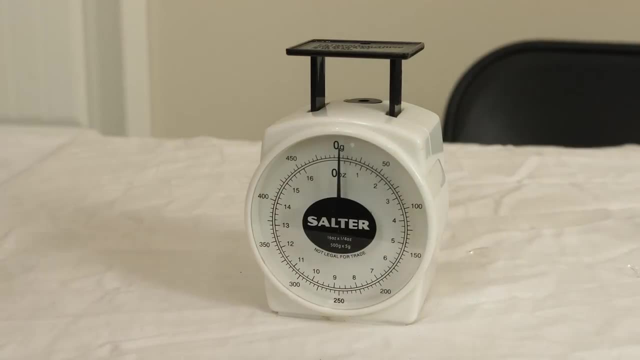 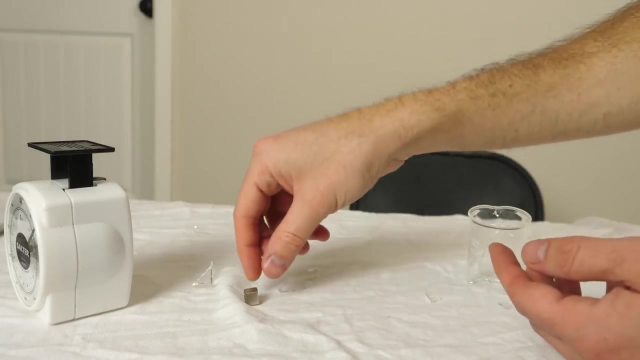 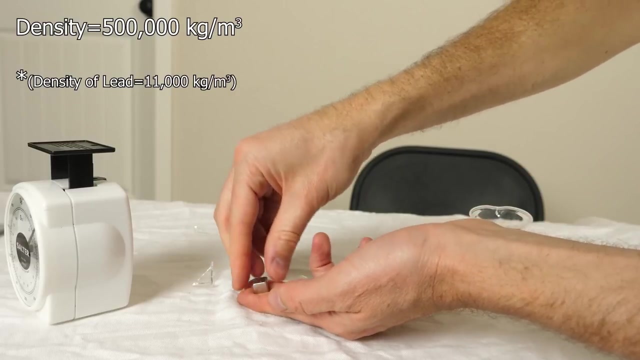 Whoa, Holy cow. Oh broke me Thing Broke through my jar. It got so heavy, Holy cow. So you can see it's extremely heavy now for the size of it. Barely pick it up. Look at that. 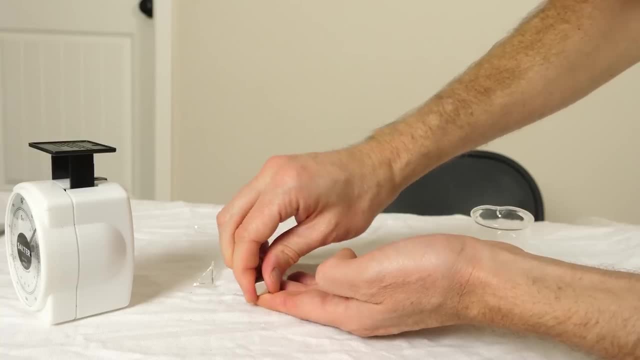 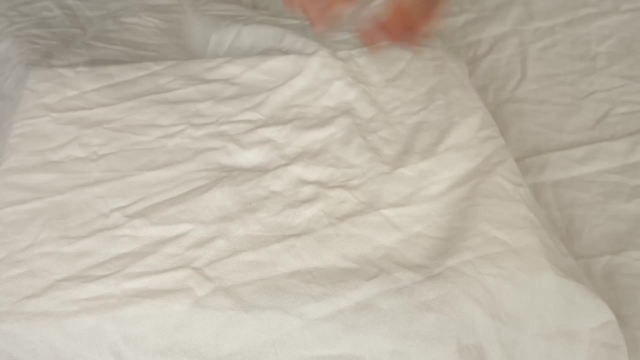 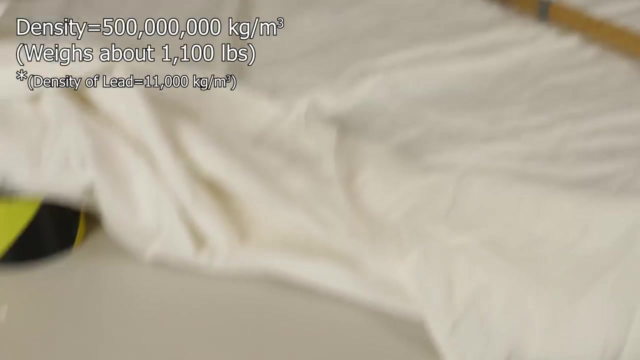 Ow. So I would say this weighs around one pound. now Can see how heavy it is here. Ow. Okay, I'm increasing the density. I can't even hold it anymore. Oh, it went through the table. Okay, so we're going to need a stronger base. 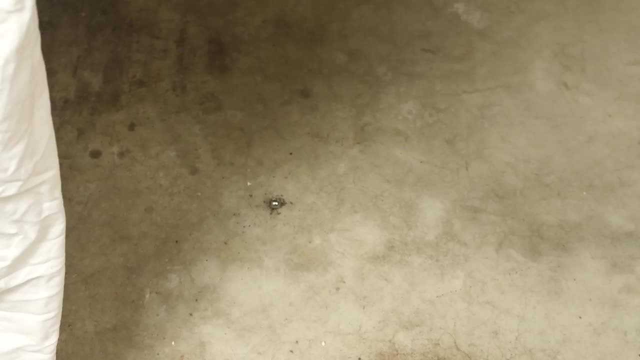 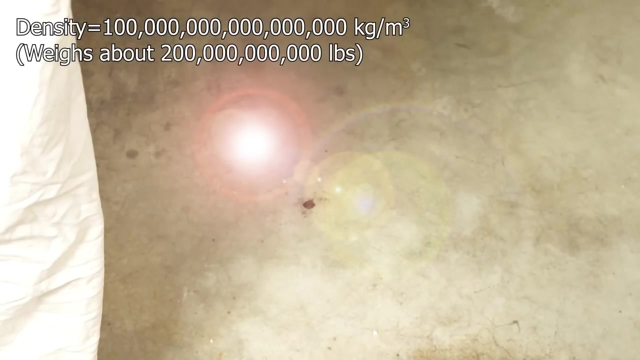 but let's just go ahead and turn it all the way up to neutron star and see what happens. Three, two, one, Whoa, It just shot through the Earth. So right now it's basically vaporizing the mantle in front of it and it is going to be getting that. 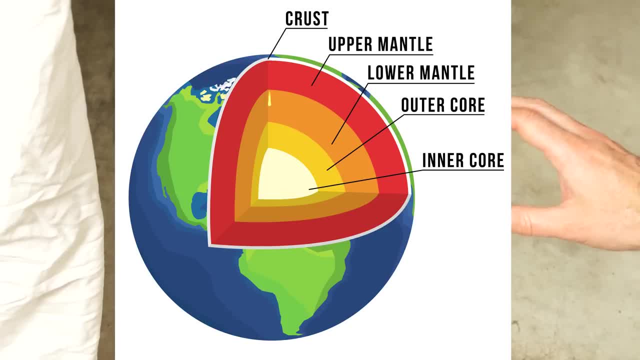 strength that it needs. So if you want to see this closer, just like that, just tap that button of it and leaving a trail of hot plasma behind it In a while as it falls, it'll eventually just become lodged in the earth's core. 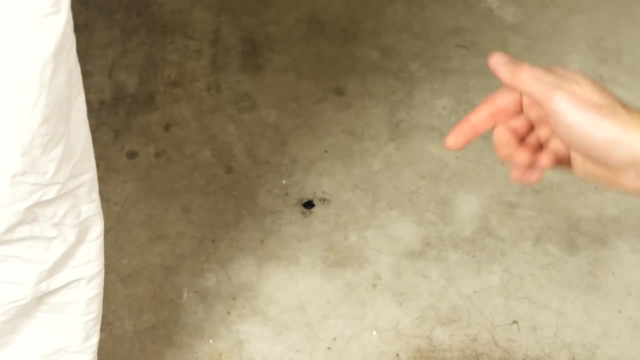 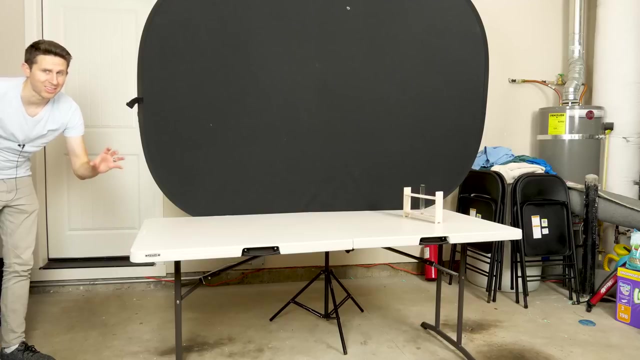 So let's try this again with a holder that will actually stop it from falling through the table and through the earth. Okay, now let's redo this experiment with a magic stand that can support the weight of the hundred billion kilograms in that tiny little centimeter cube there. 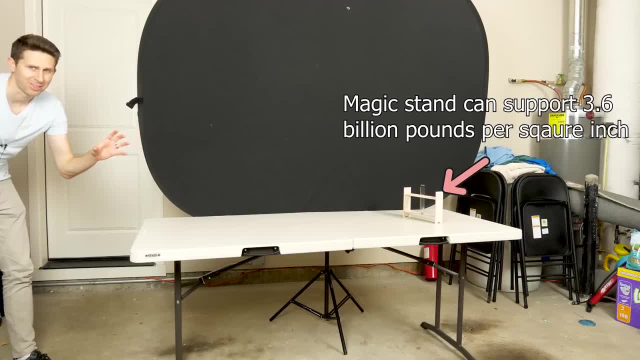 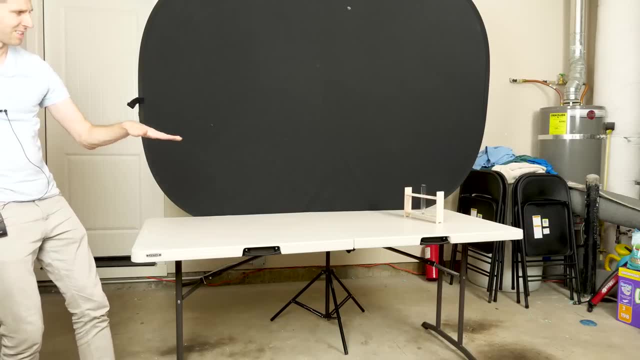 Now, because this is so dense, it has its own gravity force that I can feel. And what this feels like to me is that when I start to walk closer to it, it kind of feels like I'm starting to walk down a steep downhill because the gravity is pulling me towards. 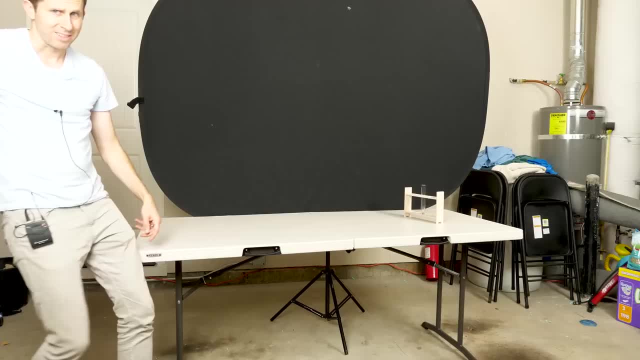 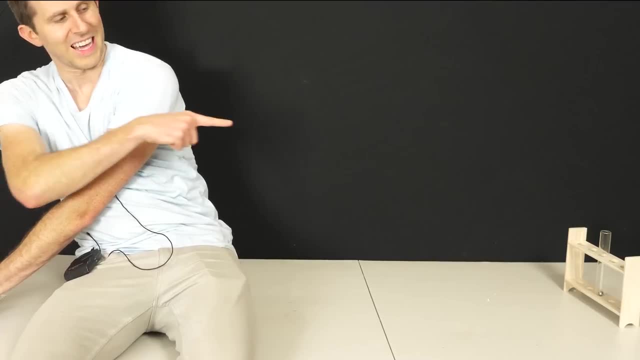 the neutron star instead of straight down towards the earth. So I kind of feel like I'm walking down a hill. So even just sitting next to it on a table, it's like gravity is pointing that way- towards the drop of the neutron star instead of straight down towards the earth. Whoa, Okay. Now because of that- Because gravity is proportional to the square of distance- it becomes increasingly hard to pull away from the neutron star drop the closer you get to it. So if you get closer than a critical distance, then you won't be able to get away from it. 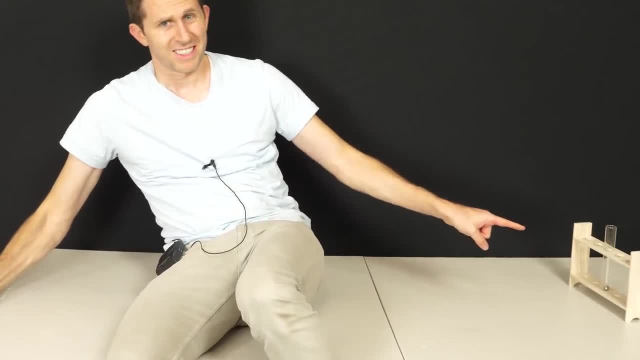 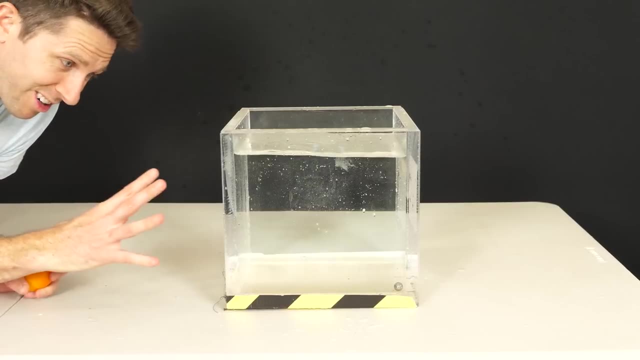 ever. So that means that if I want to touch this neutron star drop, I'm going to need another plan, And that plan has to do with water. Okay, so I managed to get some water around this, And if I didn't have this box around it, it would look like this: 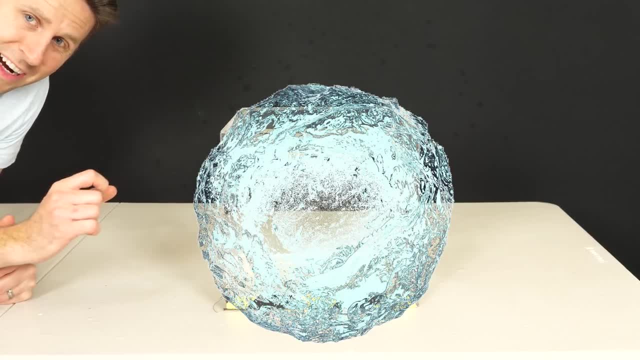 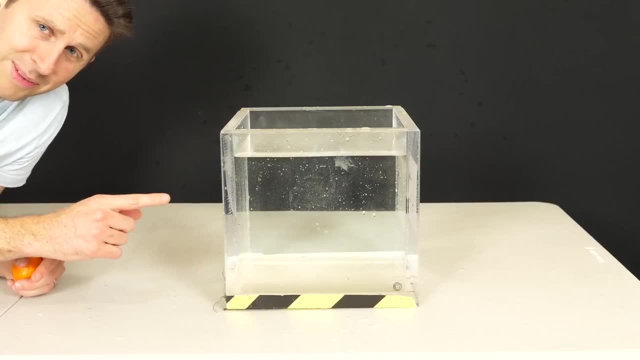 It would be a complete sphere around it, with the drop at the very center, because gravity is now pulling it all towards the center. Now normally the point of no return with a drop this size of a neutron star is around eight inches Around eight inches away. your arm would become too heavy to ever pull back and then it would. 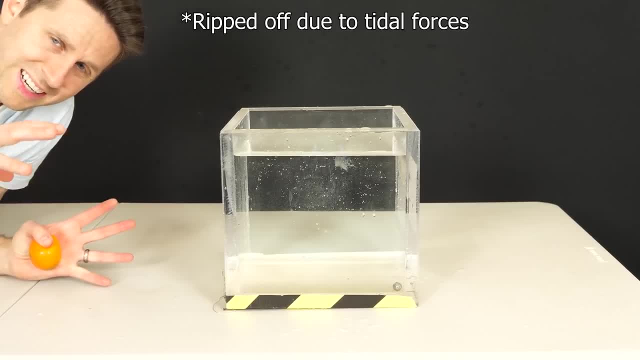 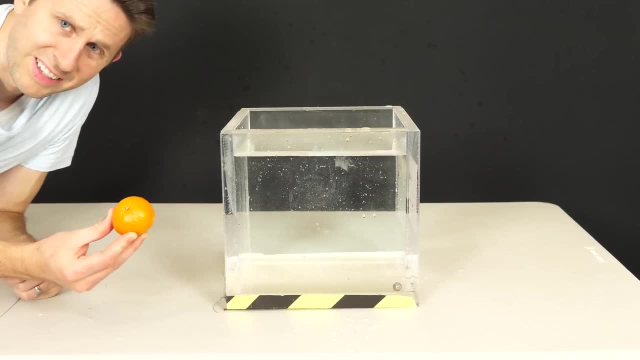 just get sucked in and probably get ripped off and it would pull your whole body in and you'd compress down into the neutron star. But if you put water around it, something interesting happens. So let's see if this orange gets sucked in. Huh. 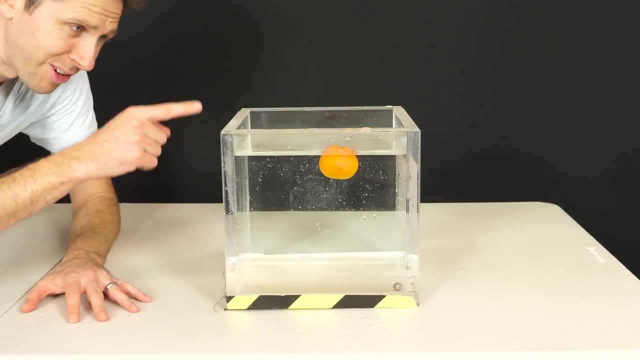 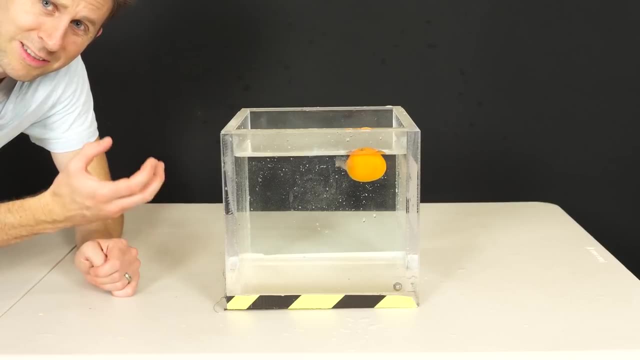 It just floats. So at this range it's hundreds of times of Earth's gravity, but it's floating on top here. So that means that buoyancy has nothing to do with the strength of gravity, And the reason it works like this is because the neutron star drop is pulling on the water. 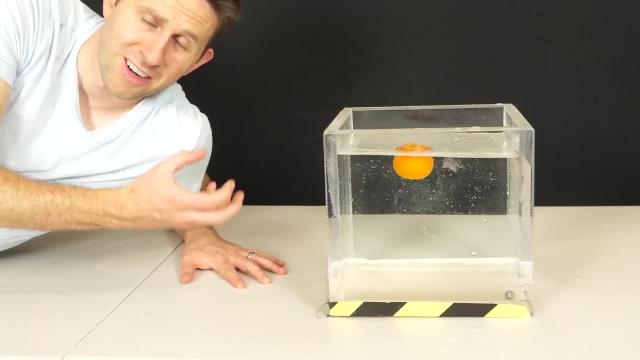 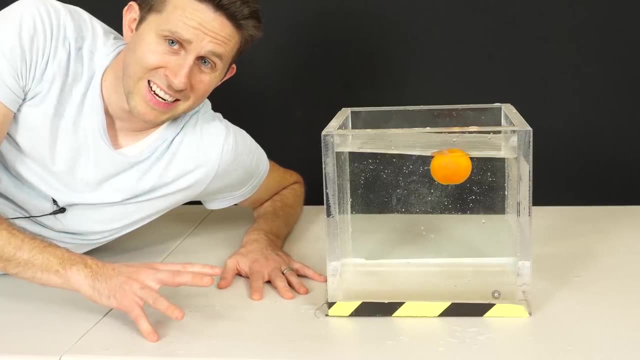 just as much as it's pulling on the orange, But it pulls on the water a little more because the water is a little more dense. so the orange still floats on top of the water. So this means on different planets, whether it had stronger or weaker gravity than Earth. 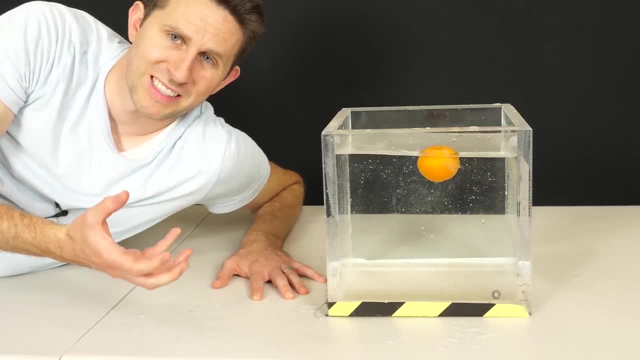 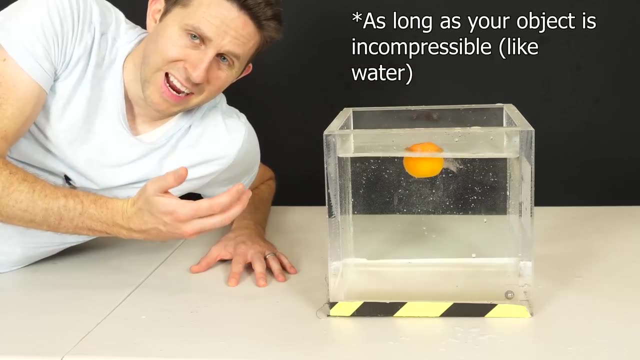 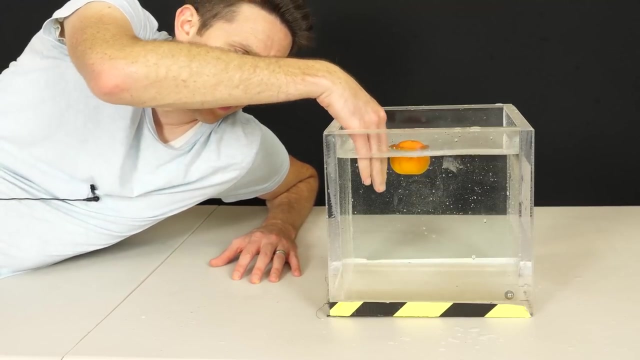 boats would still be able to float just fine. They'd have the same buoyancy as on Earth, Because buoyancy is independent of the gravitational factor. So that means my hand should be okay, because my hand is less dense than water, So my hand will never get pulled towards the neutron star stronger than water. 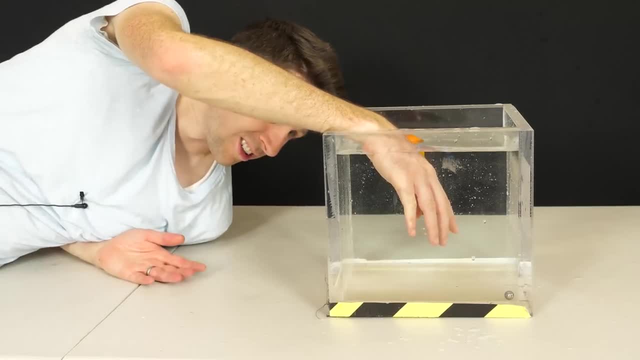 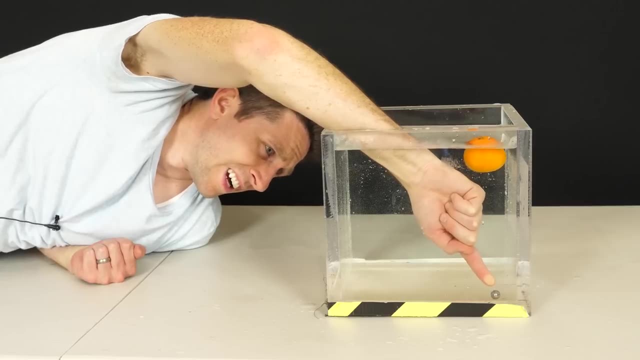 So as long as I keep it in water, I should be able to get as close to it as I can. Okay, But what happens when I get close to it is it's like there's this impenetrable layer I can't get past because my fingers are less dense than water. 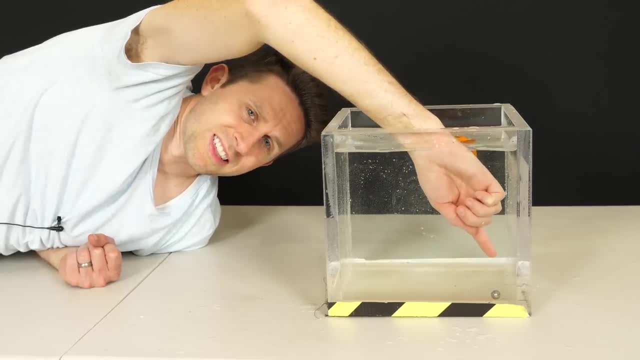 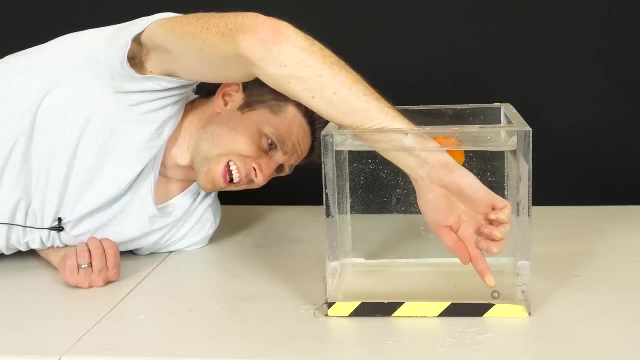 Basically, I can't penetrate this layer of water because the neutron star is pulling down on the water, no matter what, harder than it's pulling down on my finger, And so, no matter what, I can't get through the layer of water around the ball. 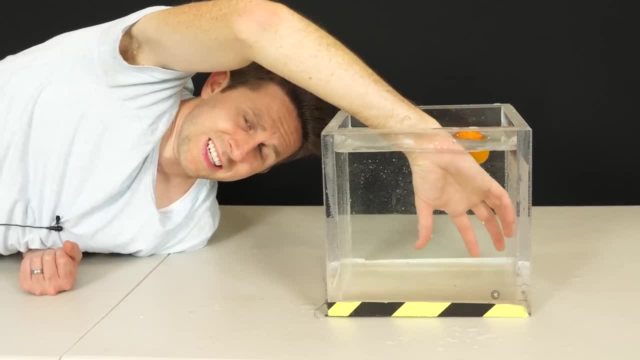 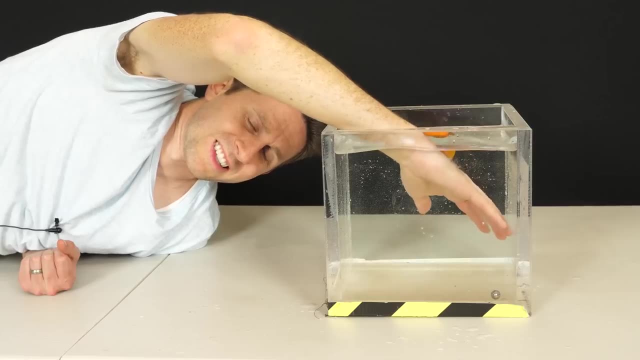 So even in this situation, even when you have water around it, you're protected from the gravity, But that means that you're going to end up with a very small layer that you can't penetrate with your finger, as long as you're less dense than water.